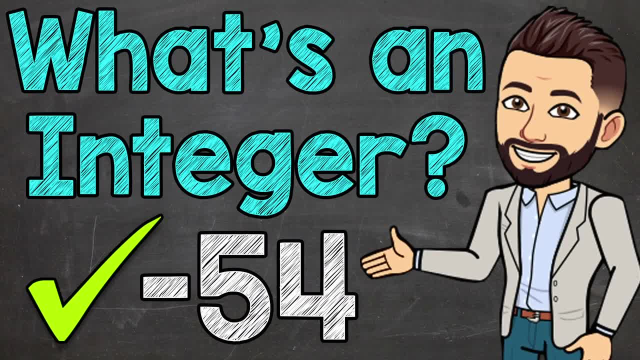 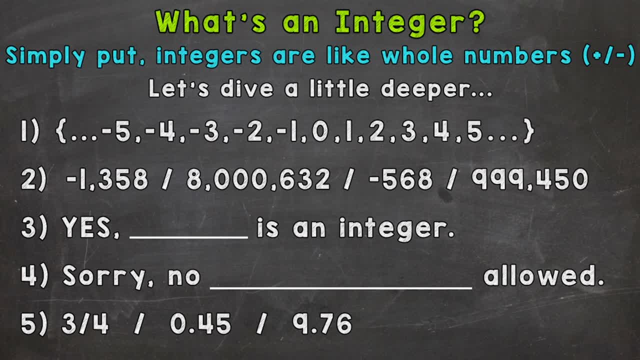 Welcome to Math with Mr J. In this video I'm going to cover what's an integer and simply put, integers are like whole numbers, but we throw negative numbers into the mix, so we have positive and negative numbers. So let's dive a little deeper in order to better understand what's an 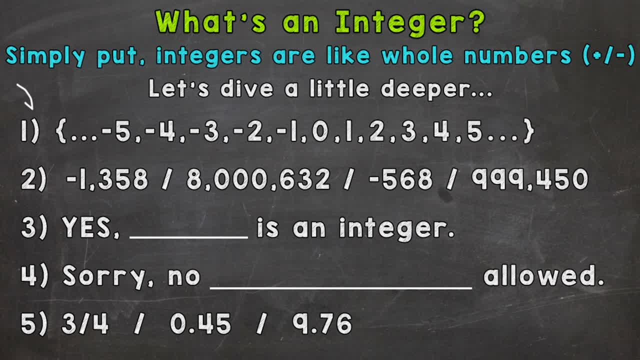 integer, So number one here, and I'll draw an arrow so you can follow along with me. we have examples of integers, and let's start in the middle, at zero, and if we go to the right, we're just counting up by one each time, so it includes. again, we have our positive integers, so one, two, three. 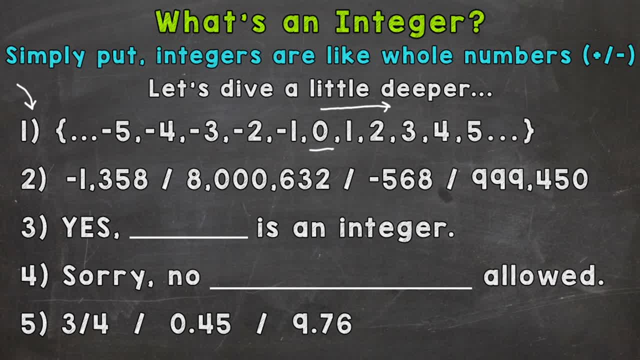 four, so on and so forth. and we also go to the left, so we go into negative numbers, so negative one, negative two, negative three, so on and so forth. So on to number two. here, where we have other examples of integers, we go further to the left of zero into negative integers and further to the right of zero to 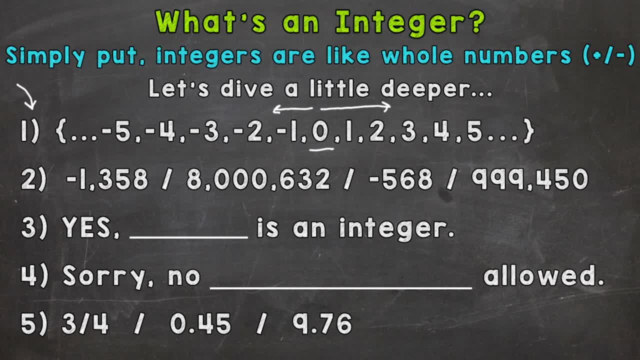 larger in value positive integers. So for the first one, we have negative 1,358. so yes, that's an integer. The second one, we have 8,632, then we have negative 568 and lastly 999,450.. So all examples of integers. Now number three is. 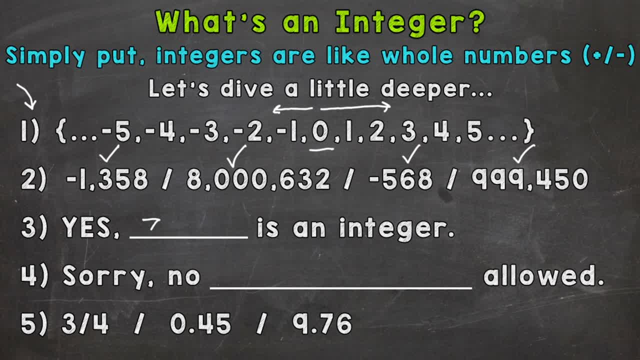 very important. Yes, zero is an integer. Number four: sorry, no fractions or decimals allowed, So fractions and decimals are not integers. So for number five we have some examples: three-fourths, not an integer, Forty-five hundredths, not an integer and lastly, nine and seventy-six hundredths. 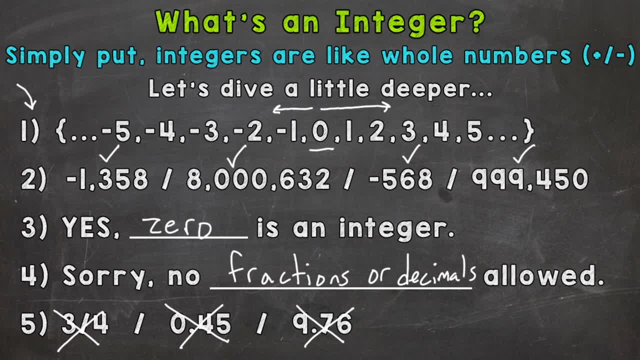 not an integer. Hopefully that overview of integers, along with examples and counter examples, help your overall understanding of what an integer is. Thanks so much for watching, Until next time, Peace.